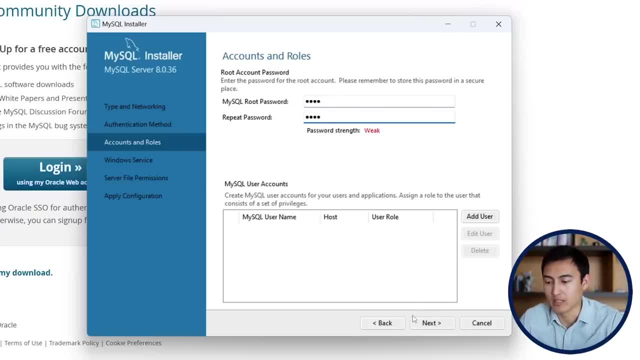 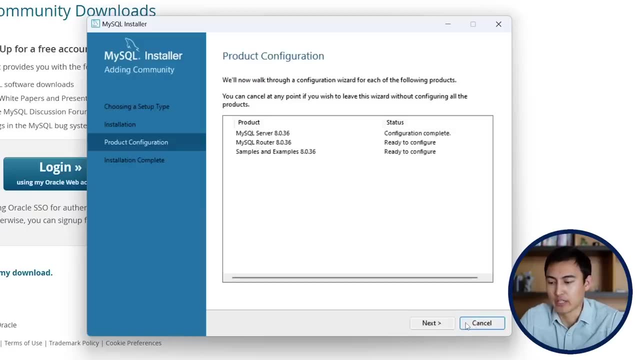 want here? I'm just going to put a simple one, Make sure you don't forget it: Click on next there, Next again, Next and execute. Now we can just go to finish there and next again. Click on finish And this: 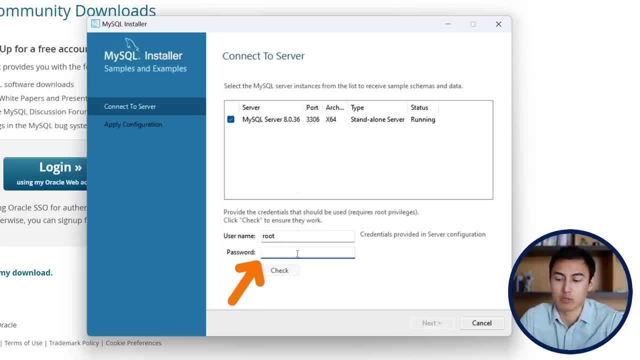 final one is going to be next, And here what we want to do is put the password that you typed earlier, So I'm just going to put mine. Click on check and you should get this connection secured button in green there, and click on next there and execute. Now we can just press on finish there and 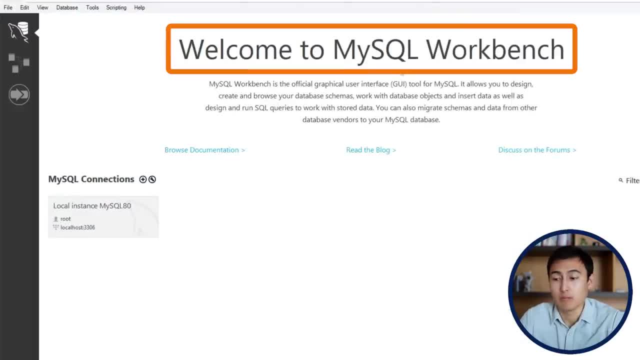 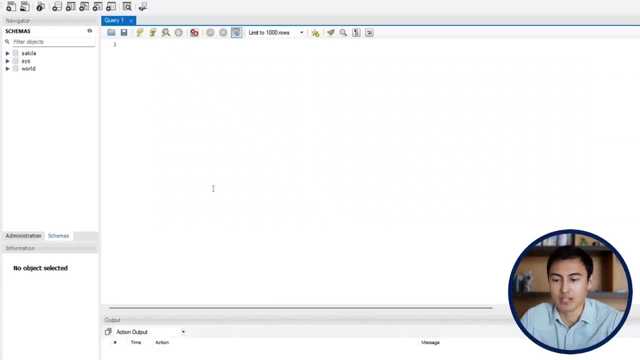 next again and finish: Awesome, This should open up MySQL Workbench, and you just want to click on this local instance, which is the one that we'll be working with, which should open up a page like this: Awesome, That's the setup process complete, And now we can go ahead and get started with the. 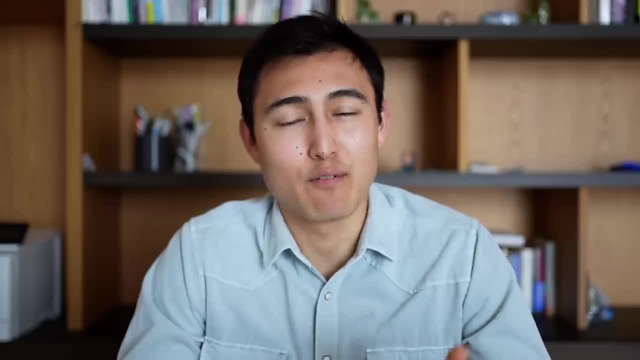 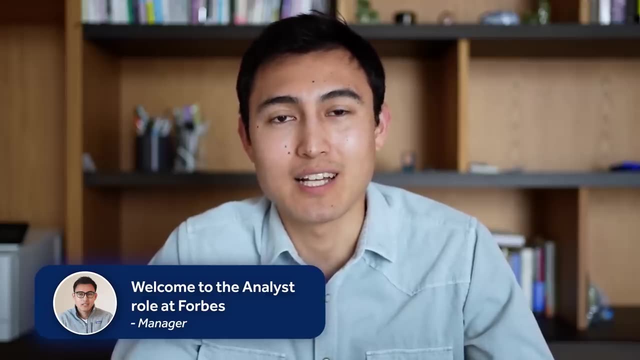 analysis. But first we need a data set to work with, And for this you can check it out in the description below. But let's suppose we're working as analysts for Forbes and they're asking us to analyze some of the trends of billionaires, So that's what the data set is about. Now, 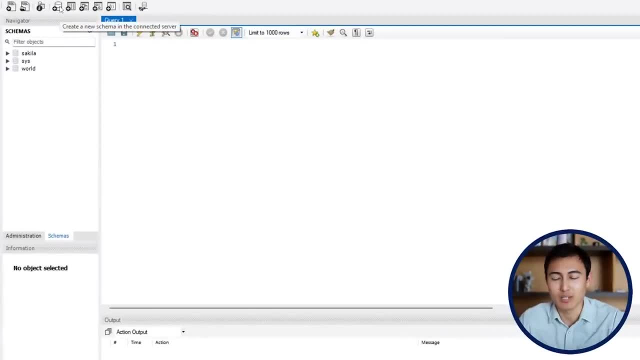 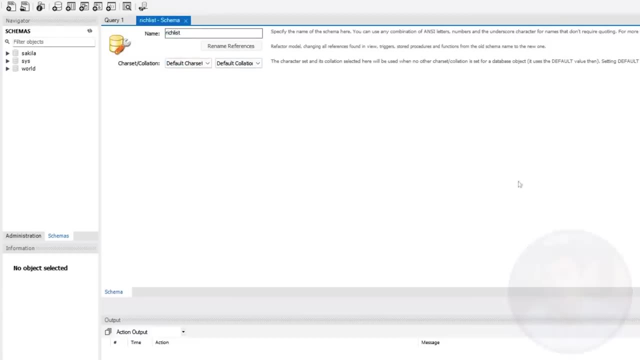 to go ahead and add it. we want to go to this button right here, Create a new Schema which is basically like a database. Let's go ahead and call this something like RichList- Just going to put it all together there- and click on Apply, Click on Apply again and. 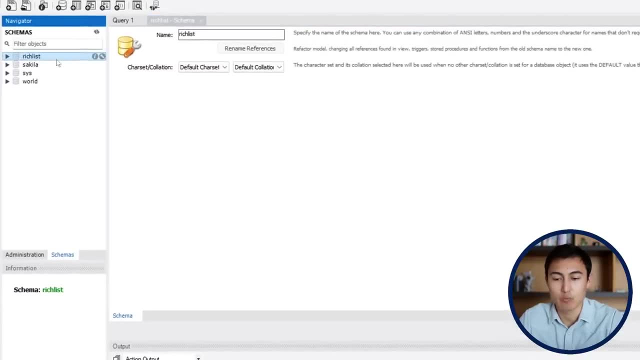 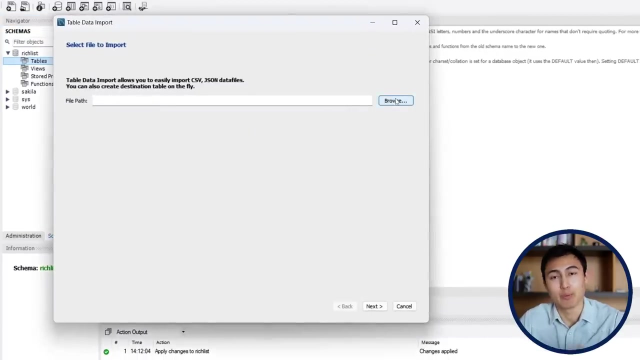 finish Now. if we refresh this on the left hand side, you can see we have this new list, which is RichList, And within it we want to import a table. to do this, We can select on tables, right click and go to table data import wizard, And here's where you would add the file that I've provided. 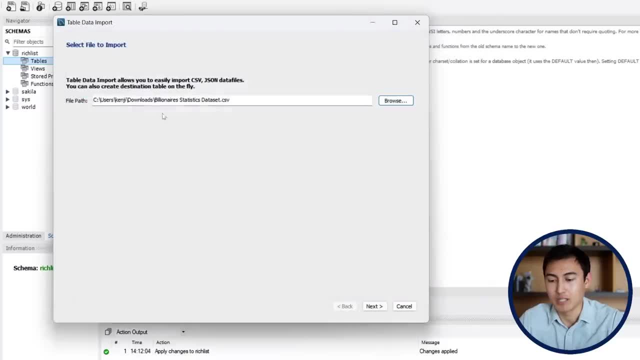 in the description said so mine is right here. i'm just going to insert it. click on next and let's go ahead and call this a new table called just billionaires, and click on next again. here's a bit of a preview. we're happy with that, so we'll just click on next. this might take a while to load. click on next there. 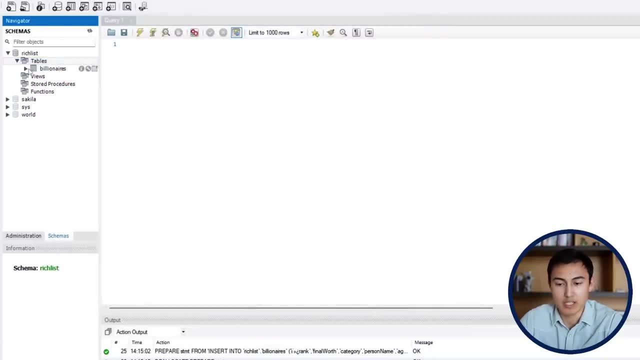 and finish now. if we refresh this over to the side, you can see we have this billionaires table and to go ahead and select it we first need to select the right database. so we can just double click on that and you can see that it's gonna turn bold. so that's how we know we have it. 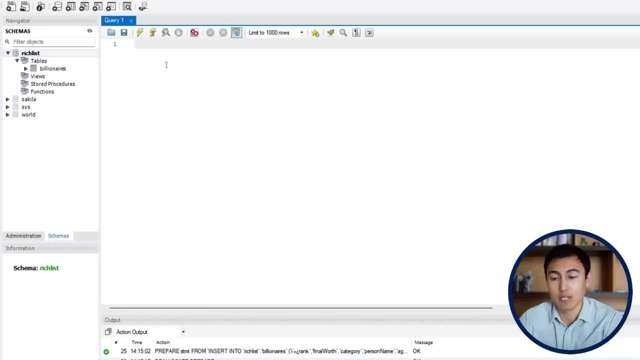 selected and to go ahead and find everything inside of that table to first preview it. we can type in here something like: select all which we can do using this asterisk from the billionaires table. right, so that's the one that we want, and we'll put the semicolon to say that we're finished. 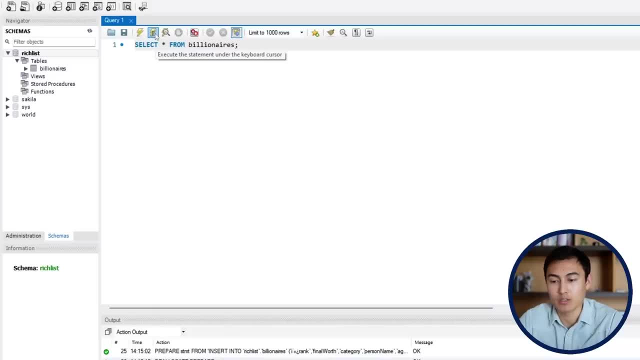 with this query and we can go ahead and run it with this thunder button so you can see. it says: execute the statement under the keyboard cursor, or we can use this other one which is executing the selected portion or everything. so we're fine with that and you can. 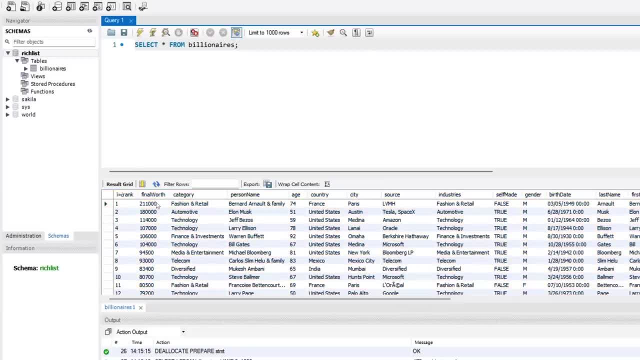 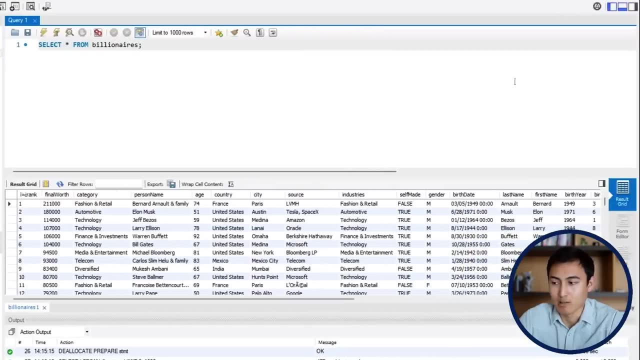 see down below what our table looks like, so we have information like their net worth, their category, their name, age and so forth. if your sql workbench doesn't look exactly the same, it could be due to these buttons over here, and you can see how you can collapse them or change them around, depending. 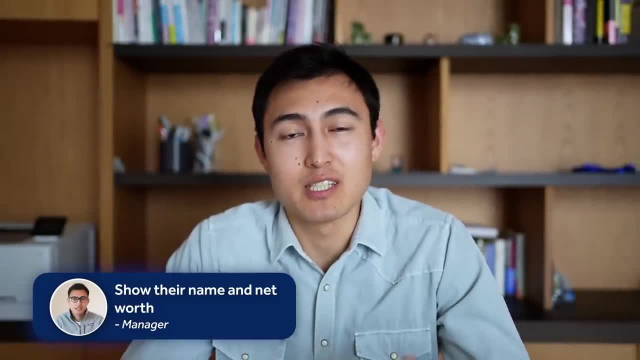 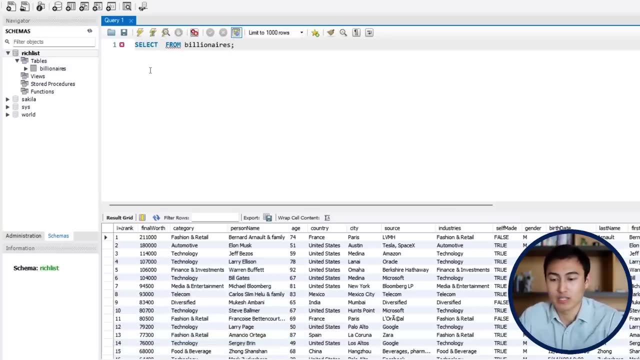 on what you want. the first task we have from our manager is that he only wants to see the person's name and their net worth. so for this, you might recall, we said select all, but instead we want to just select the person name, which is this part down here, and we also want to select the final. 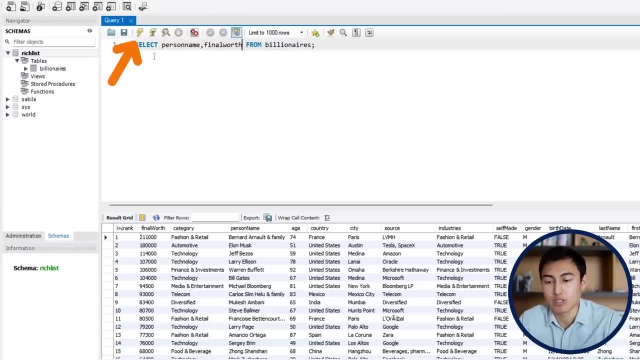 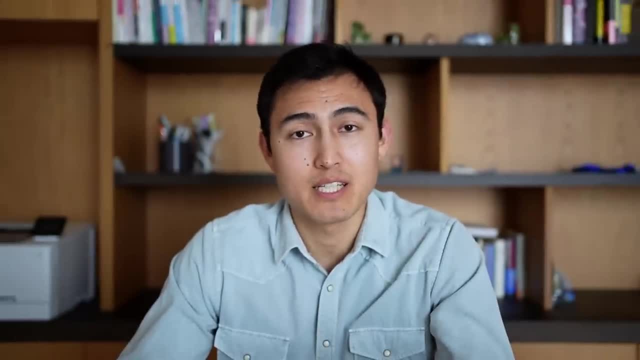 worth. so we'll put a comma and final worth and now we can just run this again and you can see right there that we have that table sorted. now that we understand these basics, let's suppose we want to find out all of the countries that are in this list. so first we can take a look at what we 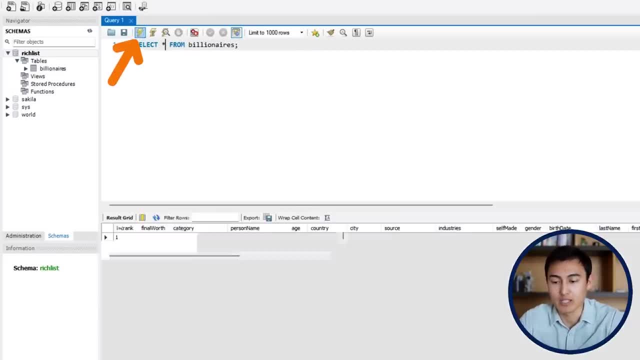 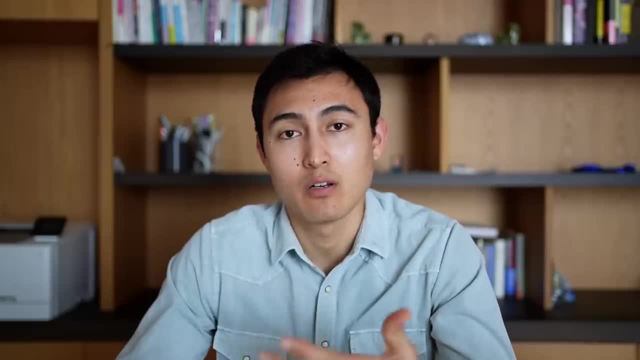 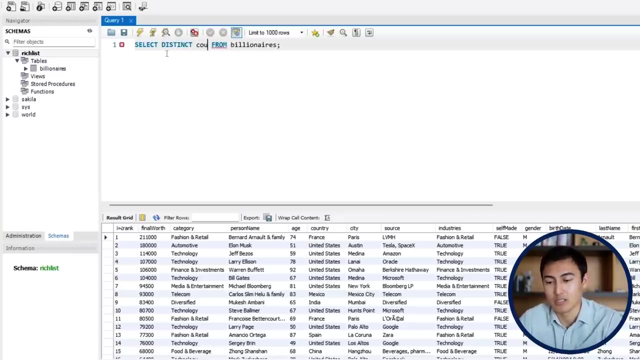 have in the whole table by putting the asterisk again and just running that so you can see we have all of the countries down over here, but there's many repeated ones, so we need to find some kind of function that works only for unique ones, so we can go ahead and put the select the distinct countries from the 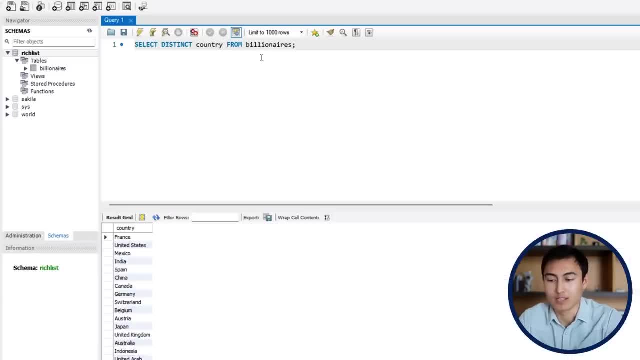 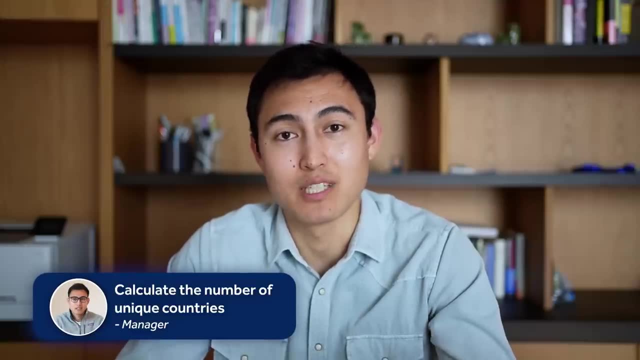 billionaires table and now we can run that. you can also hit ctrl, enter there as a shortcut and you can see. we have all of the unique list. that said, our manager wants to know the count of these, so what's the total of the countries that are in this list? and we can see that we have all of the. 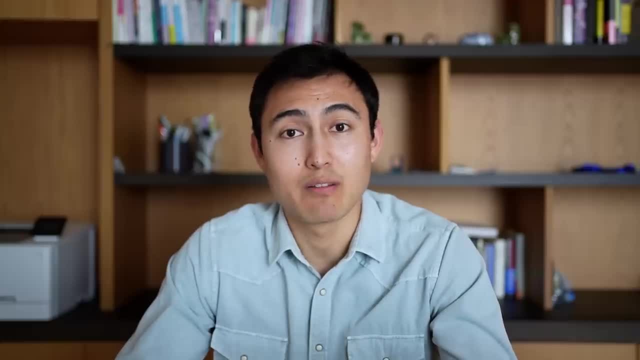 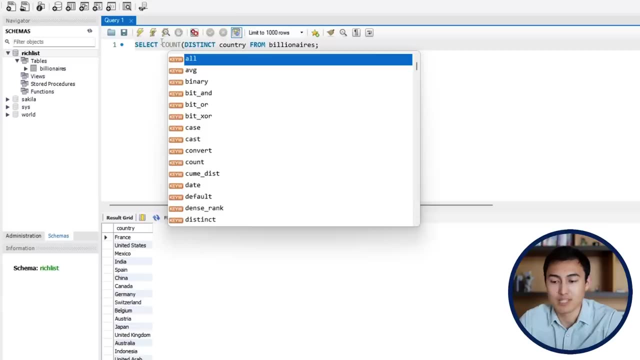 number of unique countries we have. well, that's where aggregate functions come in, and we can use that by putting a count up in here. and what do we want to count? well, all the distinct countries. so we'll put those in parentheses there, like so, and now we'll run that and you can see we have a count. 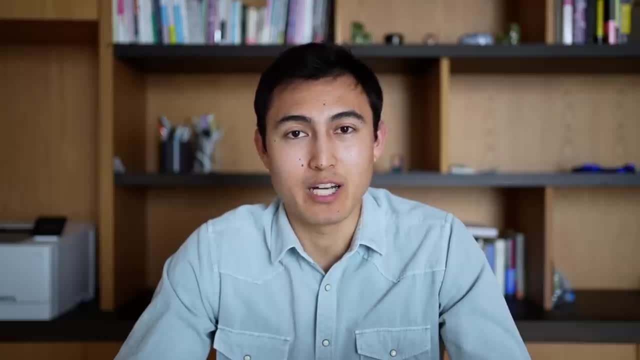 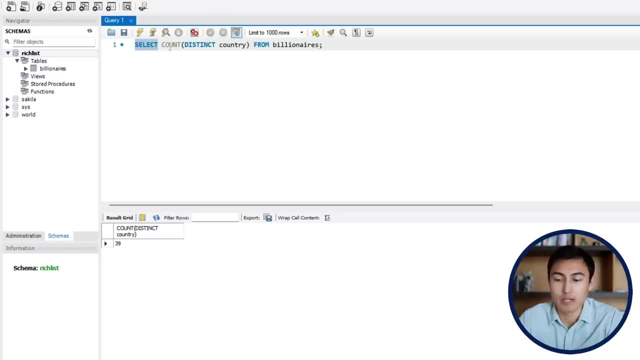 of 39 countries. at this point you might wonder why we're capitalizing some words and the overall interface is not case sensitive. that said, generally when it's in sql you might capitalize everything, while if it's just text, you would put it in lowercase. that's how you would distinguish. 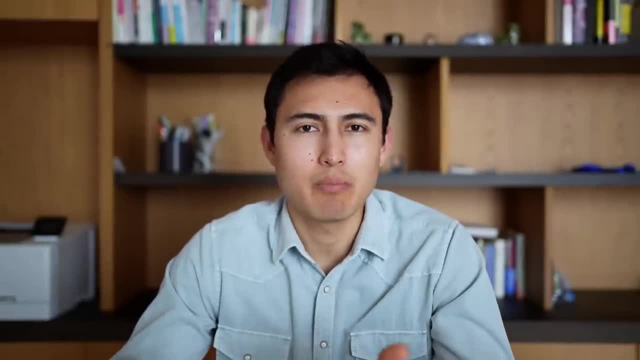 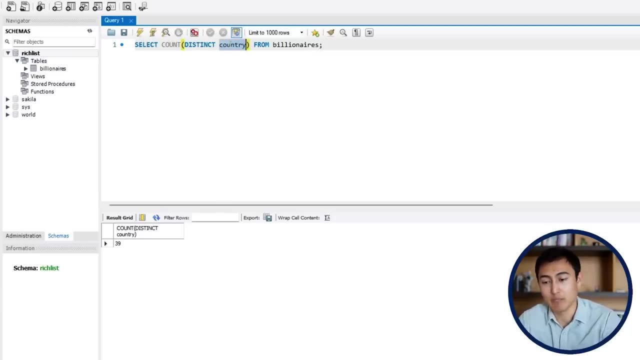 between the two. so we know there's 39 countries, but how many people are actually in this list? well, for that, it's selecting the count of distinct instead of country, it's of people, right? and if you might recall from here, if we hover and click over it, you can see we have all of the column names and 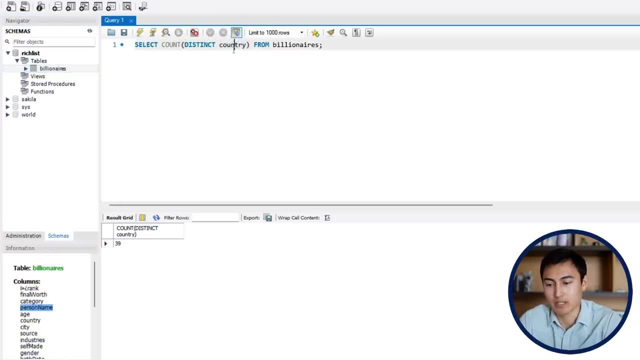 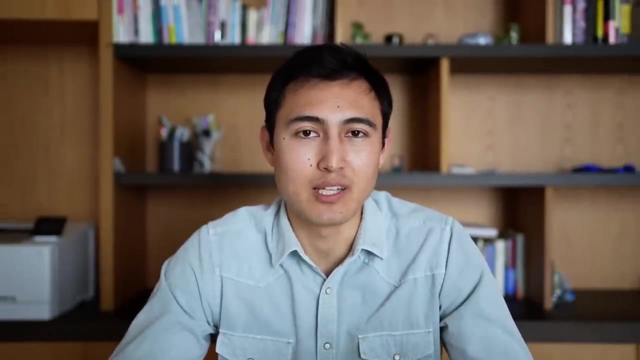 the one we're looking for is the person name, so we can type it in here just as person name and control it. control enter. so you can see we have roughly 500 people in this list. continuing on with aggregate functions, it would be interesting to see what the average net worth is of this list. 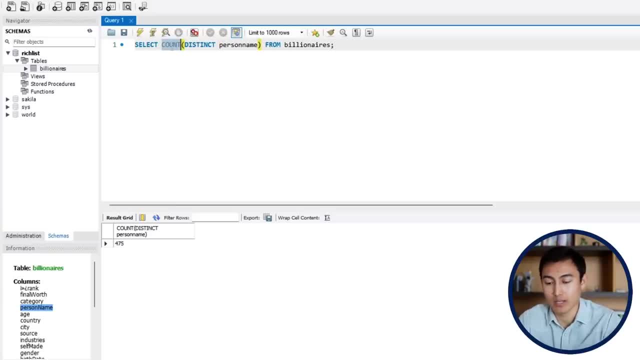 so for this, instead of a count, we're gonna go with an average which we type by typing avg, and so it's going to be the average, not the distinct person name, but rather the average net worth, which is the final worth from the billionaire's table, and we'll hit control, enter and you. 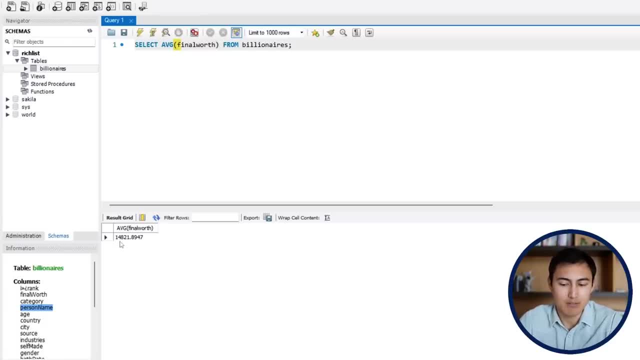 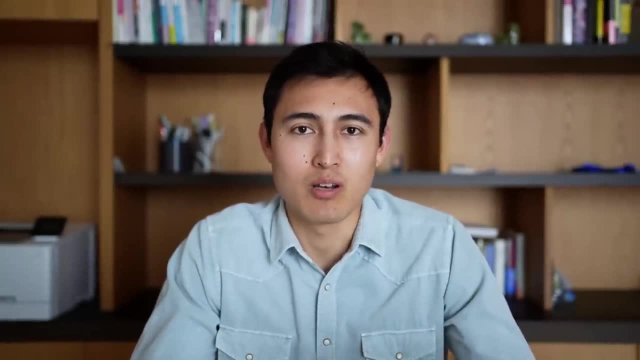 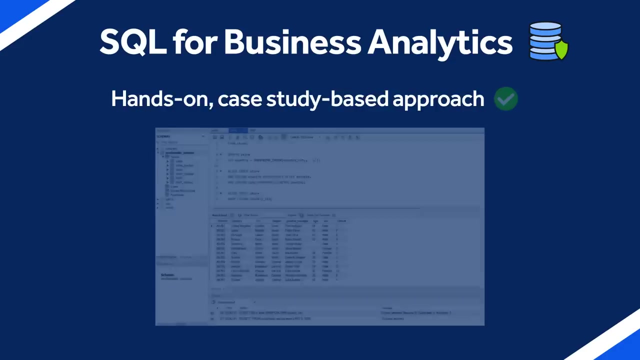 can see that I think this. these figures are Millions, so it's an average of 14.8 billion. if you're liking this video and the teaching style and you want to invest into learning sequel, you can consider taking our SQL for business analytics course with our hands-on case study based approach. 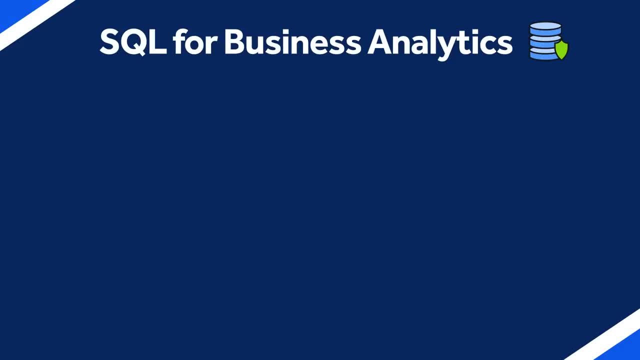 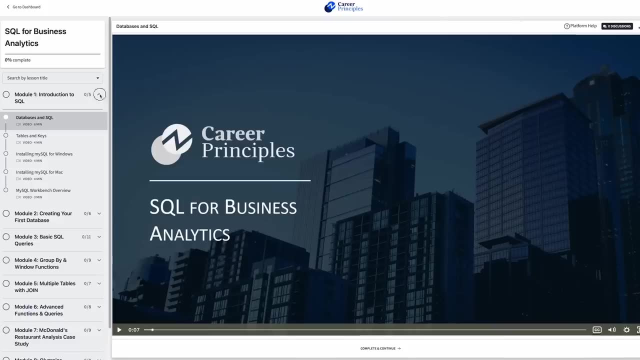 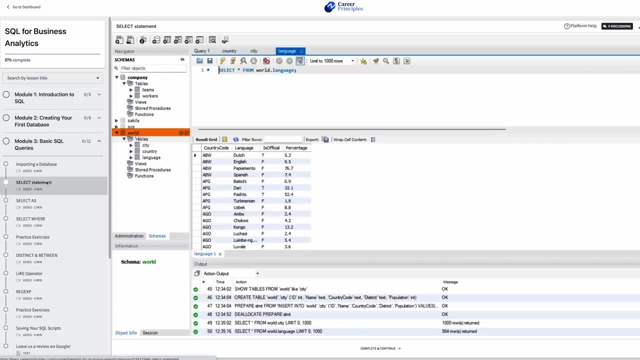 to learning sequel. you'll go from complete beginner to confidently adding this skill on your resume and using it on the job. our curriculum starts with the basics of databases and get started with sql. from here you'll learn to create your own databases, add tables and values inside of it. then you learn to interact with the database by writing queries from very simple. 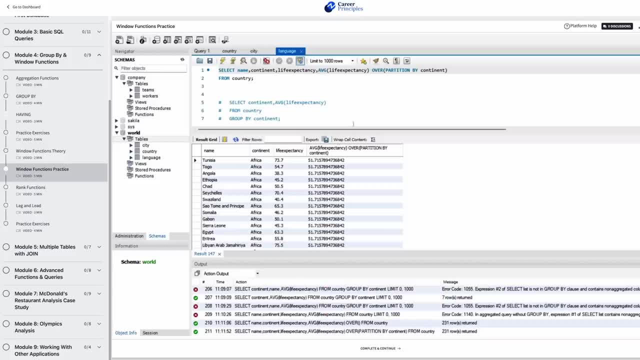 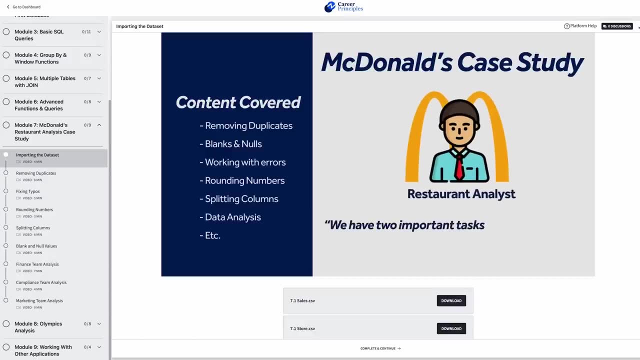 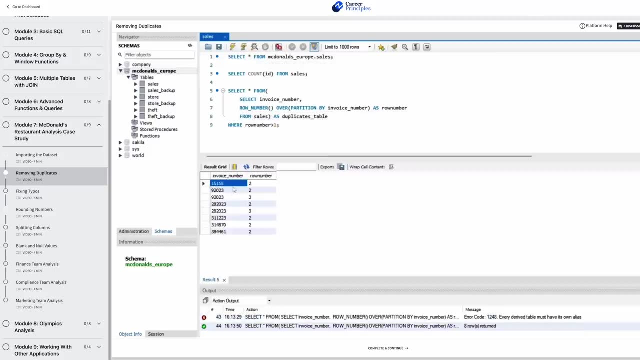 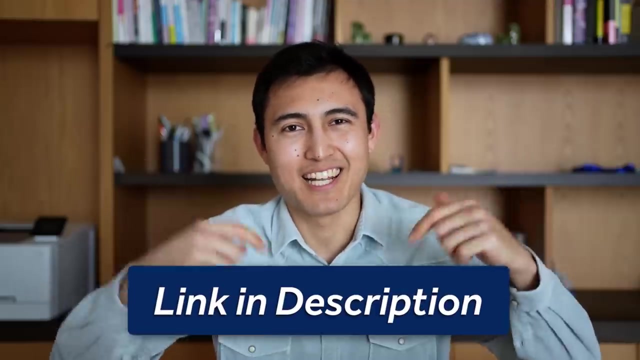 select statements to more complex window functions, joins and even sub queries. finally, once you're comfortable with sql, we'll work on two extensive case studies designed to simulate a real-world scenario where you'll be working as an analyst, both cleaning up data and extracting valuable insights based on your team's requests. so if you're interested, check out the link in the. 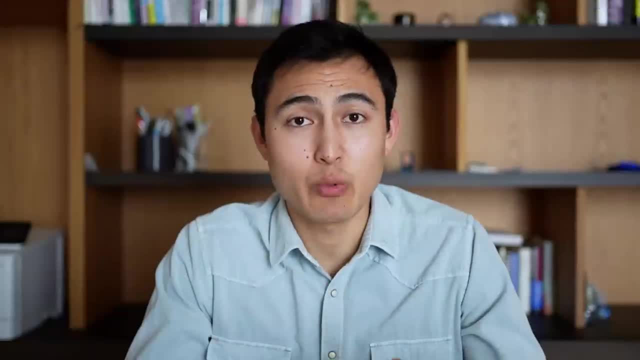 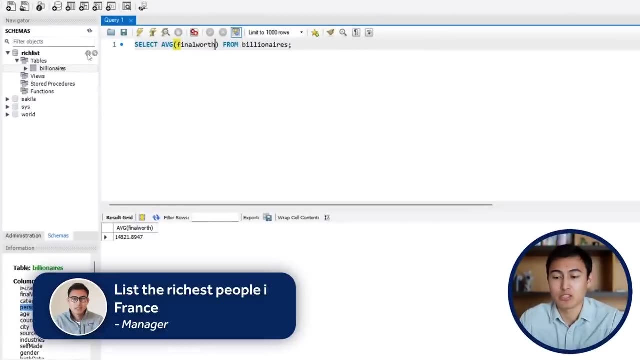 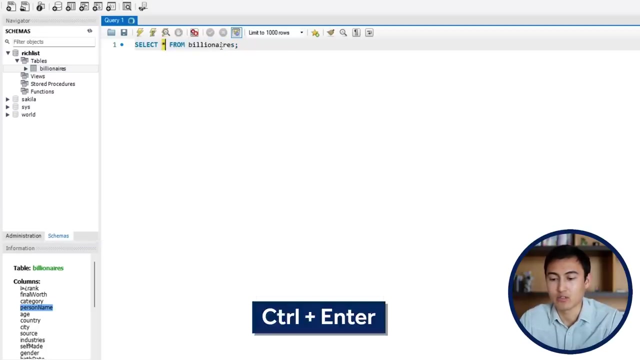 description below. alright, back to video. now that we understand the basics of the select statement and aggregations, we can start to filter. for example, suppose our manager is asking us for the richest people in france? well, for this let's go back to select all first and hit control enter. 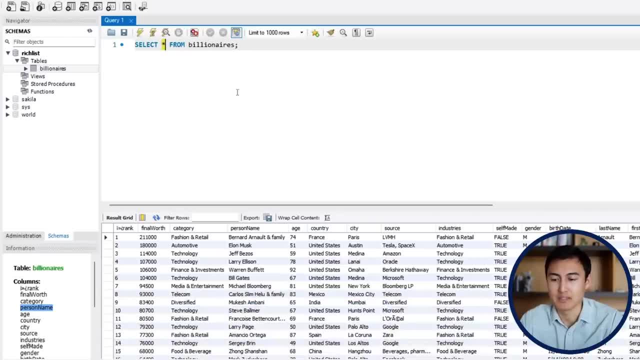 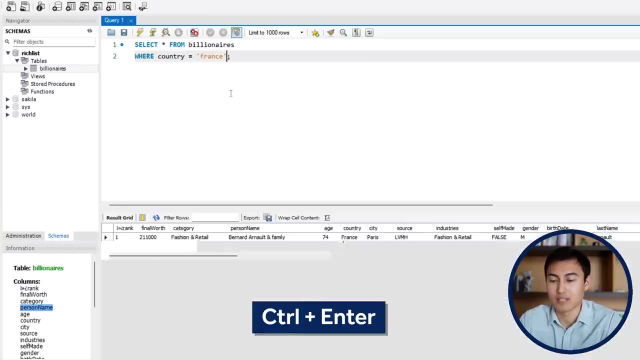 and we want to find the country that's only equal to france, right? so select all from billionaires and we'll just hit enter here where the country is equals to, and we'll put it in these quotes here: france, and now hit control enter again. so this should now be a list that's only france. 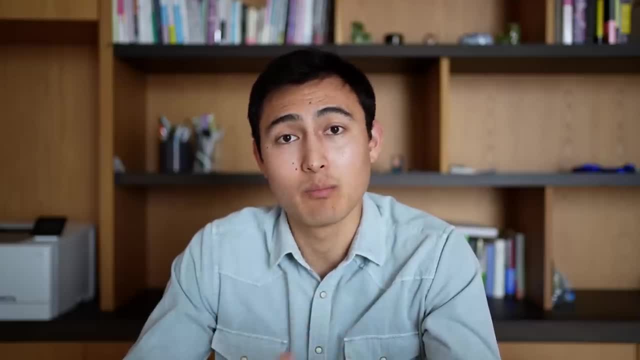 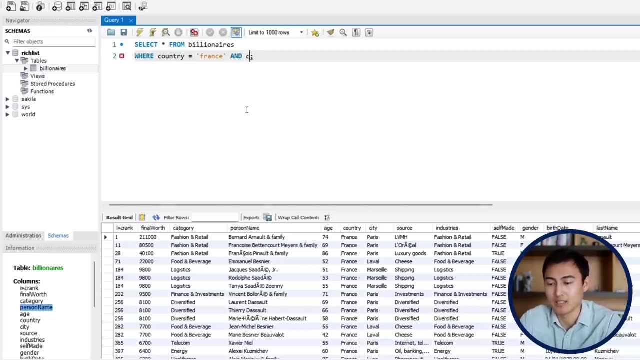 that said, that's only one condition at the moment. we can add multiple conditions. let's suppose that it's france, but it can't be in the city of paris. so we can say: and there the city is not equals, and for this we use this sign right here. 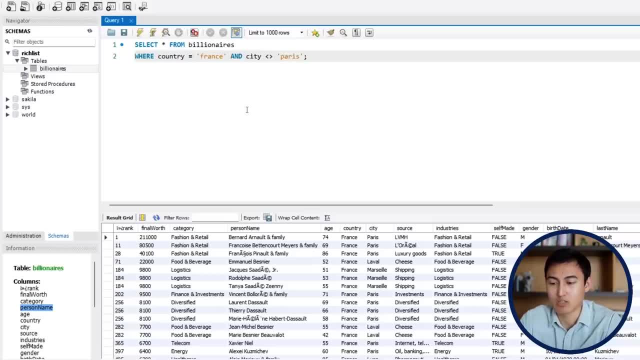 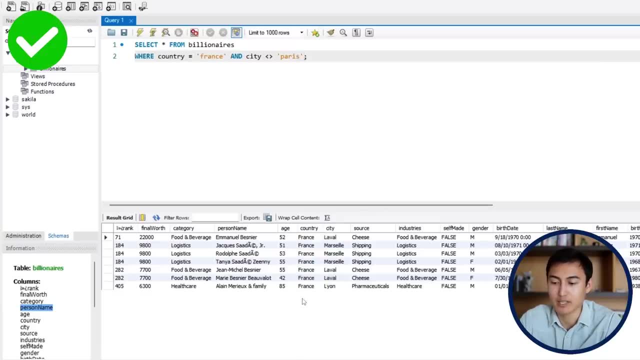 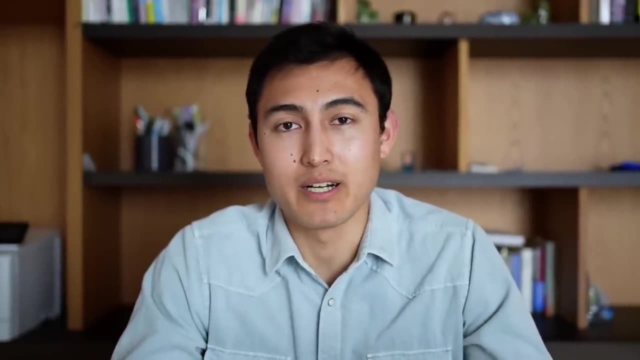 to in quotations there: paris. let's close the quotations and control enter again so you'll see all of these billionaires here are not from paris, but they're still french. you can see, there we filtered with the and condition. we can also filter with the or, for example, people that are in france or in spain, so we can switch the and there to an or. 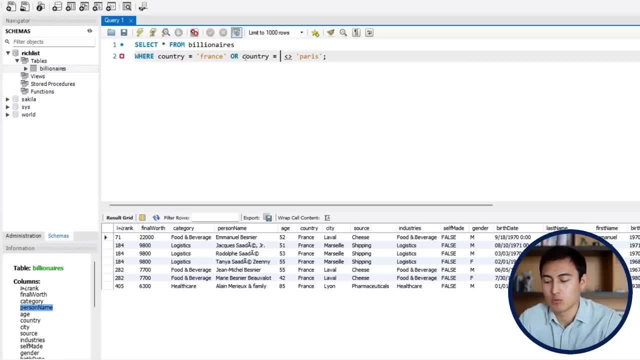 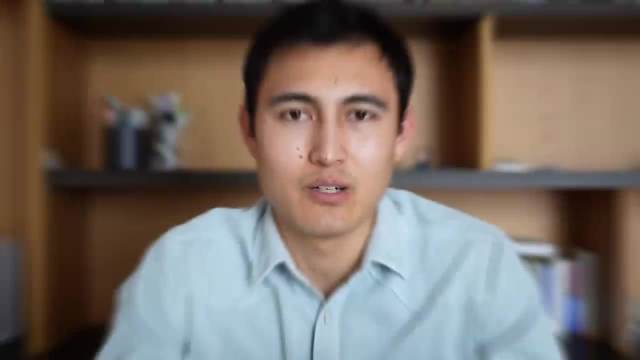 the country again is equals to in quotes. there let's say spain. so now we're saying where the country is equal to france or spain. let's go ahead and run that one and you can see there that we get some people from france while others from spain. right now we only have 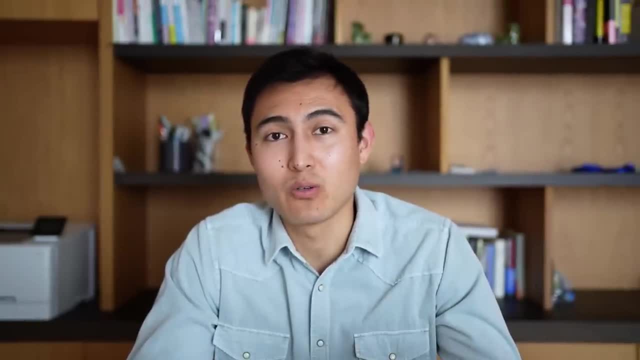 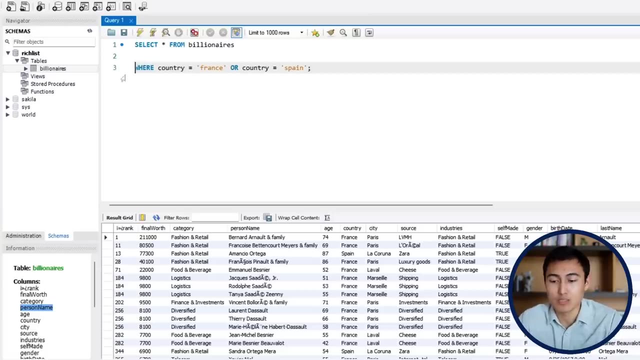 two options: france or spain. we can also add an other, or, but when it comes to multiple conditions, it's sometimes easier to use the in, so let's take a look at that, and for this we can always comment this part out. maybe we want to reference it in the future just by using this sign over here. 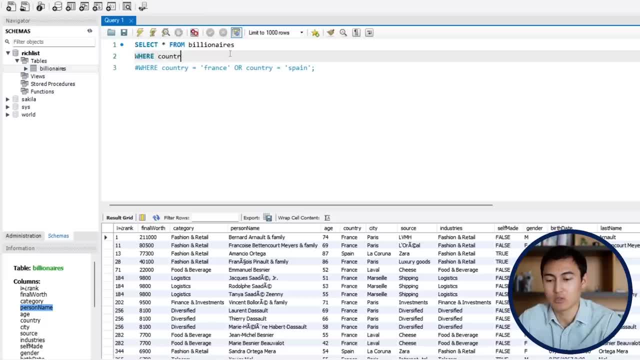 you can see that the color changes, so where the country is in and in parentheses here we can put all of the countries we want. let's say one is france comma, then let's say we also want spain comma and finally we want italy. you can see, i'm putting all of those in quotations. we'll close. 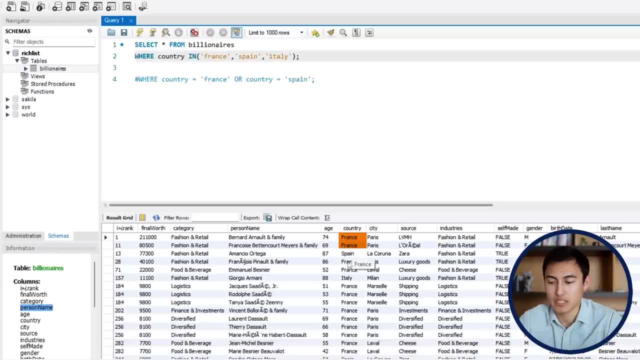 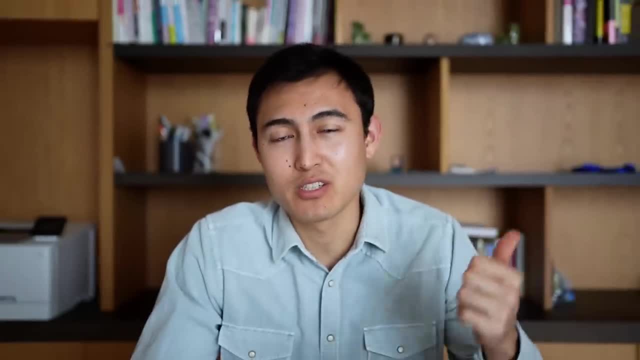 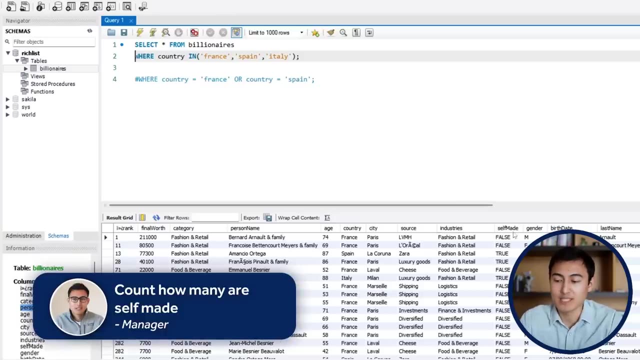 the parentheses, and now we can just run that part. so you can see, we get some people from france, some from spain and even some from italy, and here we now know aggregate functions and we also know the filtering, so let's try to combine these two. for this our manager is asking out of this list. 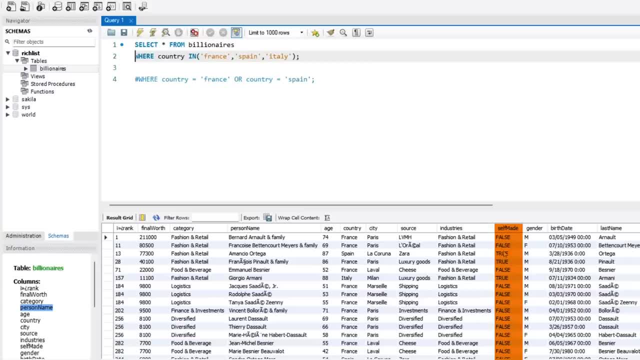 count how many are self-made. you can see that column down over here because we're counting it's going to be. let's say we put it down over here. select the count of person name. so it's a count of all of the people from the billionaires list. 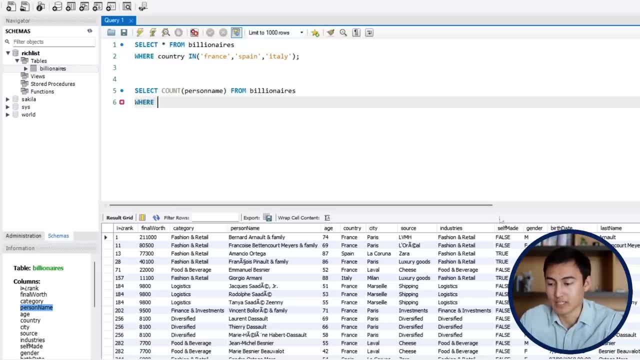 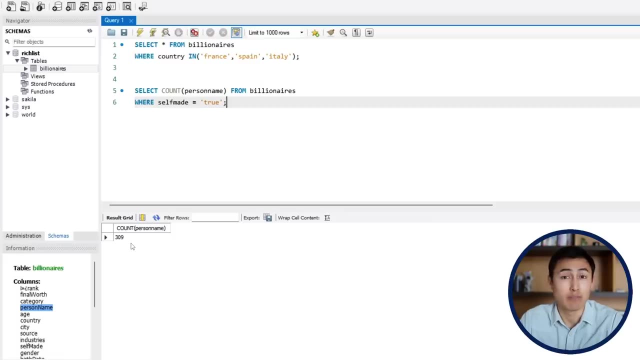 where under the self-made, so self-made table. if they're equal to true, so those people would be self-made. basically, let's try to run that part and you can see here that around 310 out of roughly 500 that we had are actually self-made. next up, our manager wants us to find the number of 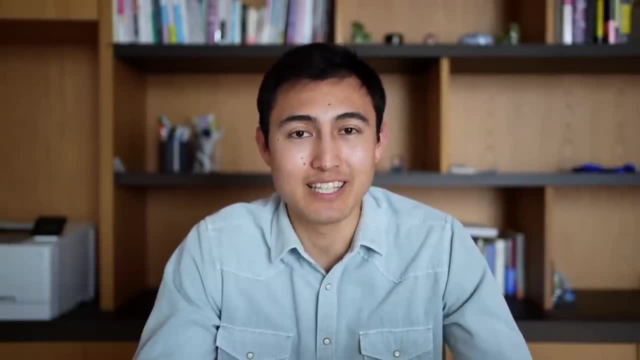 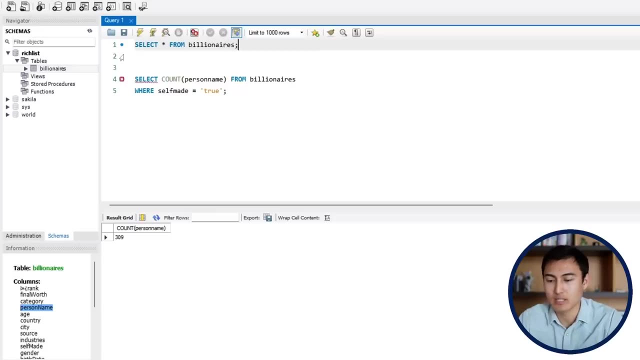 billionaires by industry. this is where we'll need to use the group by statement. so let's take a look at that. after all, we are grouping, but first i'm just gonna delete this part and show the whole table so we can get a better idea. you can see down here we have industries, so we're gonna want to get. 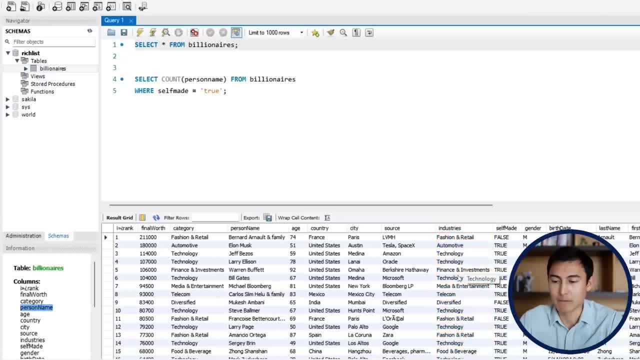 the count of billionaires by industry. so we need two things. one is going to be industries comma- let me just delete this part so you don't get confused there- so industries- and the other one is going to be the count of person name from the billionaires table and we want to group this right. so it's going to be: group by what are we grouping by? by all the. 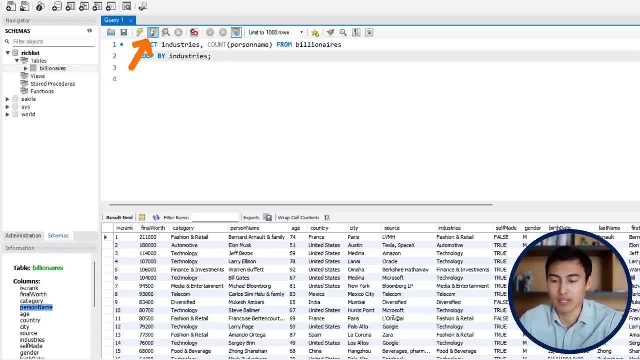 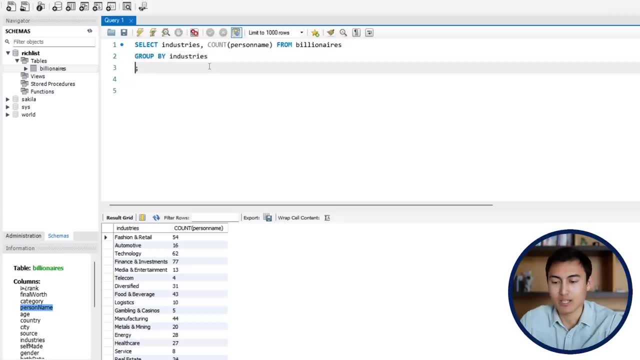 different industries. right, and now we can just put the semicolon and run that so you can see. here we get the full breakdown, but it's not in any particular order. let's try to add an order by. so. we want to order by the count, so by this column right, which is the count of the person. 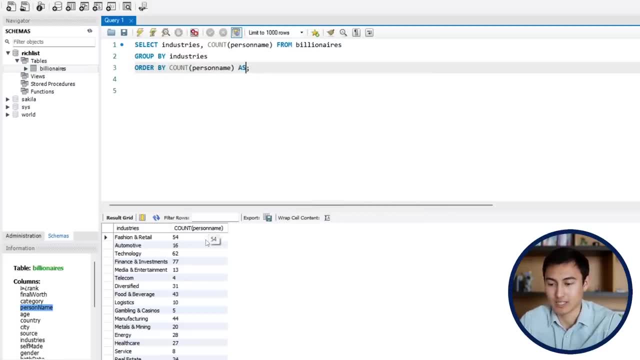 name, and we can order it either in ascending or descending order, which would be from high to low. so let's try that, and you can see here that the industry with the highest billionaires seems to be finance and investments. that said, the count of person name isn't a very nice header. 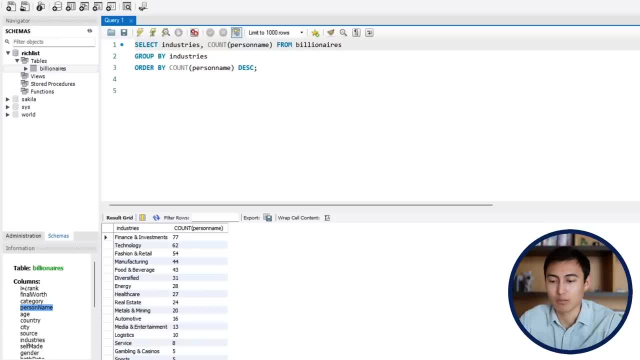 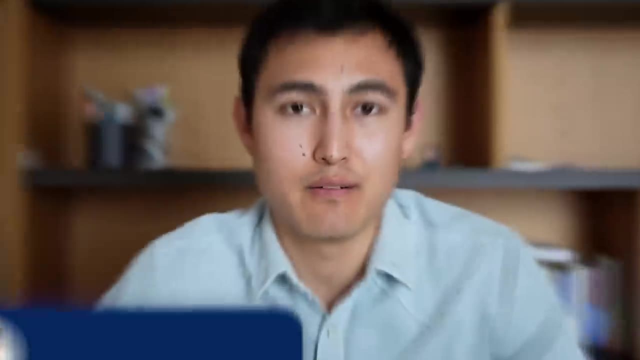 so maybe we can change the header name for that. we first put it up here so we can just change it to an alias, so count of the person name as something like billionaire count and control, enter. you can see how that's changed, that header name. finally, suppose our 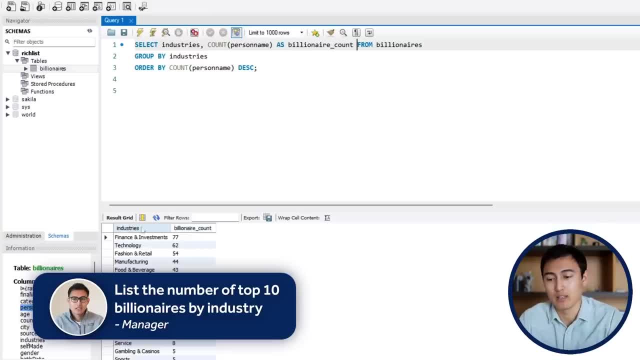 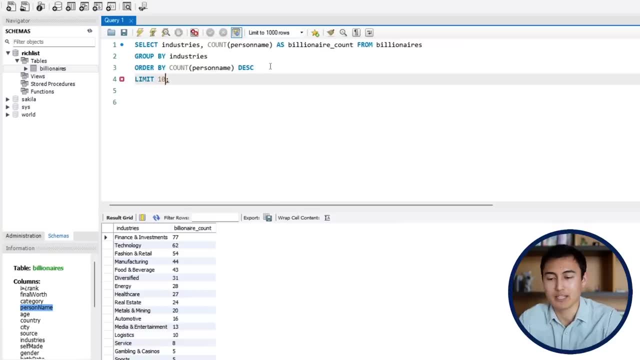 manager wants to cap this table at the top 10. only for that we can put what's known as a limit, so the very end there. i'm going to put a limit to, let's say, 10 people and i'm just gonna run that. now you can see we only get a list of 10, and this is fully dynamic, so i can always change to 15. 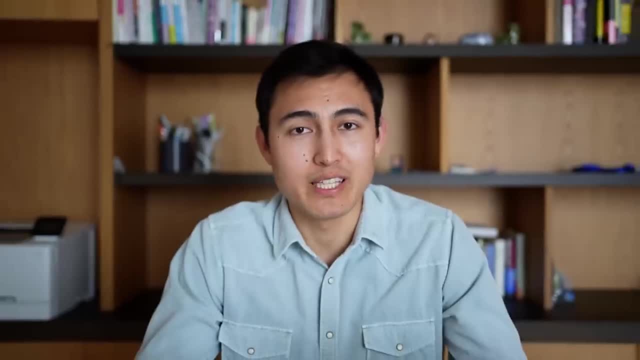 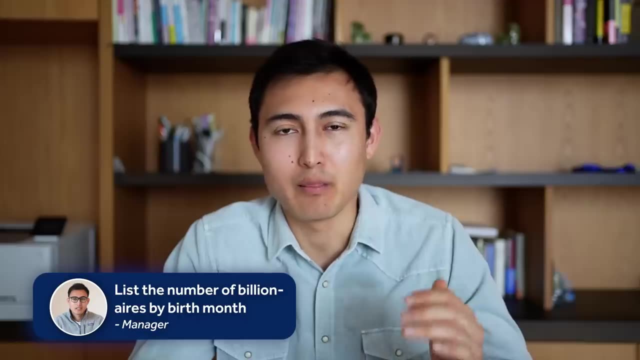 and it's gonna update fairly quickly. now that you get the idea, let's practice with another one. and suppose our manager is asking for the number of billionaires by birth month. he's maybe thinking that some people born earlier in the year have a higher likelihood of becoming 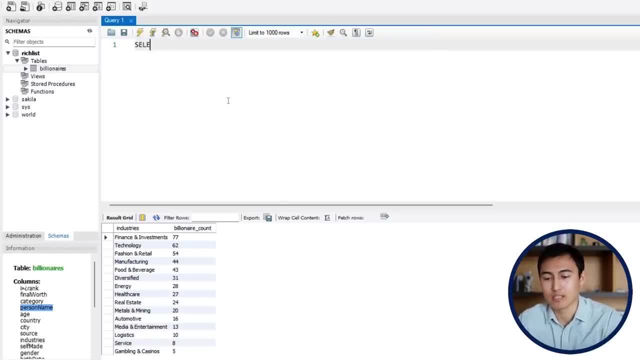 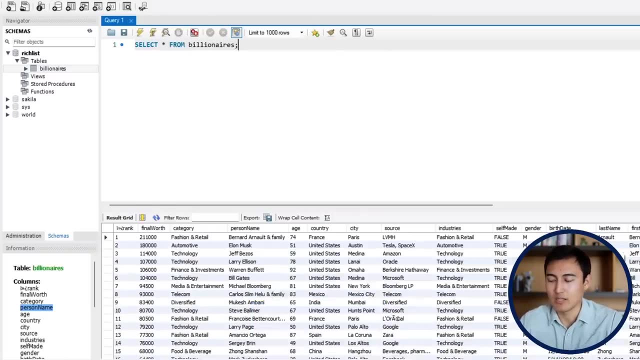 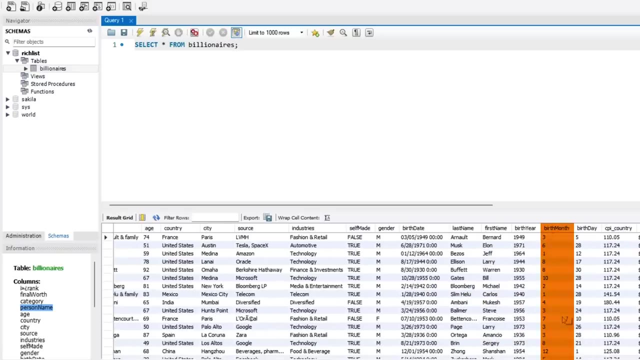 billionaires. so first let's go ahead and delete all of this and we'll just put select all from billionaires and just control enter. so you can see, if we scroll over to the side, we have what's known as the birth month. so that's going to be what we're going to be grouping by, and feel free to. 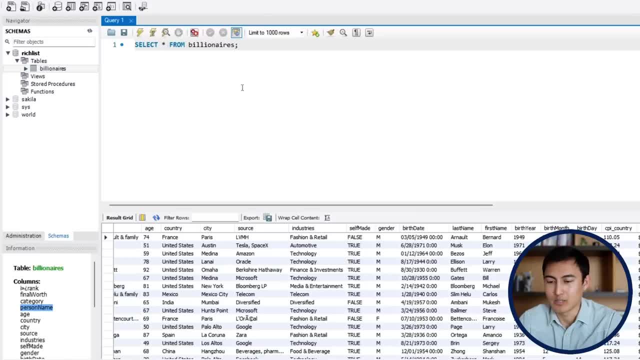 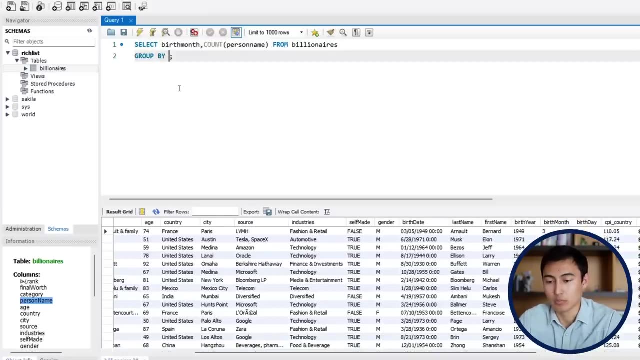 pause this video and give this one a try on your own, all right. so it's going to be to select one: the birth month comma, and two: we're also going to select the count of the person name. that's how we'll know how many to put in each group from billionaires, and we want to group by the birth. 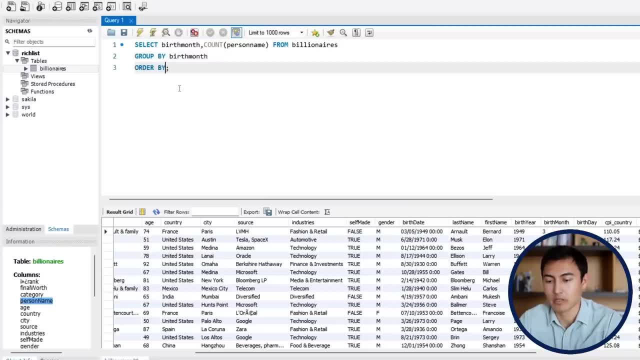 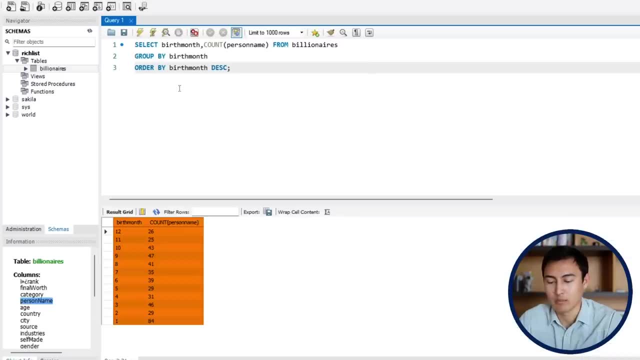 month and let's also order this already. so order by birth month in the sending order. let's try run that see what comes up. so actually maybe it makes more sense in ascending order and control enter so you can see there that in the month of January we actually have the highest number of billionaires. 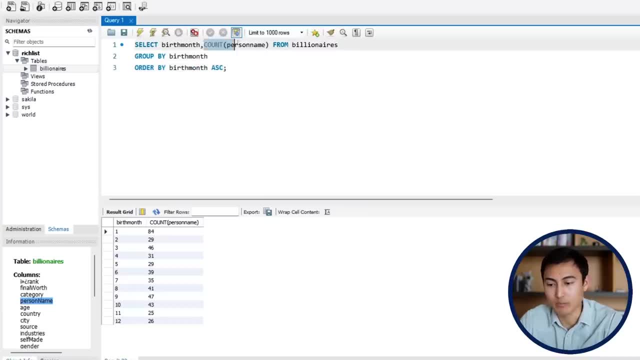 even better. instead of ordering by birth month, we could order by the count of personal name. so let's go ahead and put that in here and control enter. and instead of ascending, let's put it in the sending order and control enter. so you can see January is the highest, followed by September. 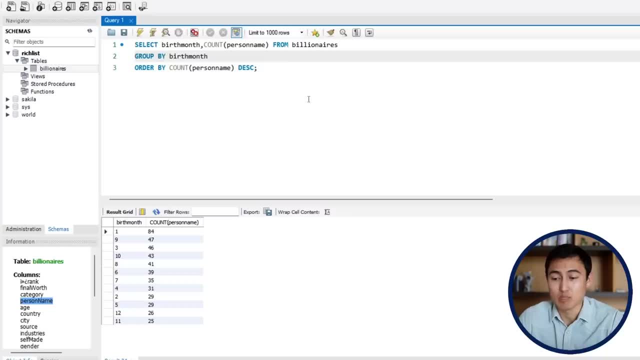 finally, let's talk about saving and exporting, and let's suppose that this is a very big query. it took you a long time to make and maybe you want to save it. we can do that by pressing on this button, so we want to save the script to a file, and you'll notice here that it. 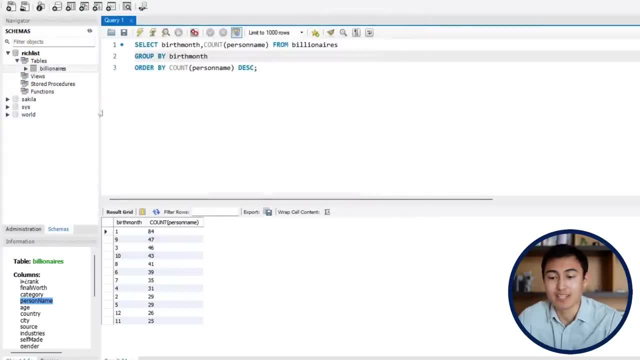 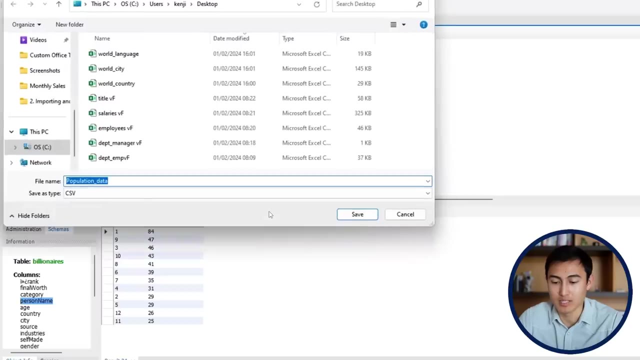 saves as a dot sequel and if we were to save it and then open it up, it would show up exactly like this again. similarly, suppose we want to export our results. you can see them down over here. maybe we want to take this table into Excel. we can just click on the export button over to the side and 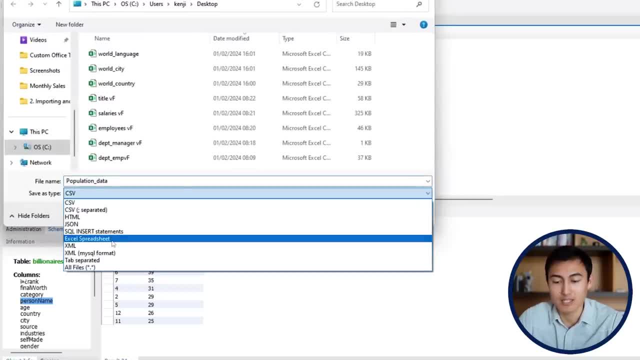 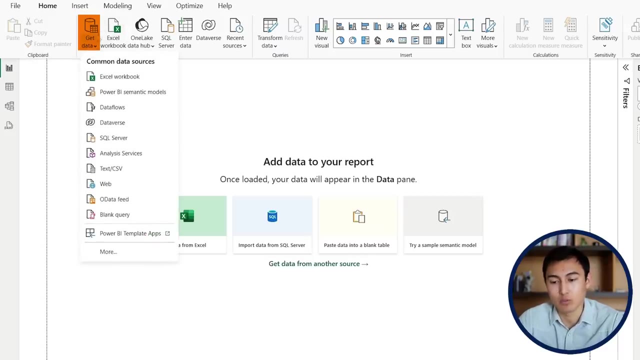 you can see here that we can't save it as a CSV as well as an Excel spreadsheet if we wanted. for now I'm just going to save it as a CSV. let me call this billionaires and click on save. here I am in power bi and let's suppose I want to import all of that data, so I'm gonna go to get data and text. 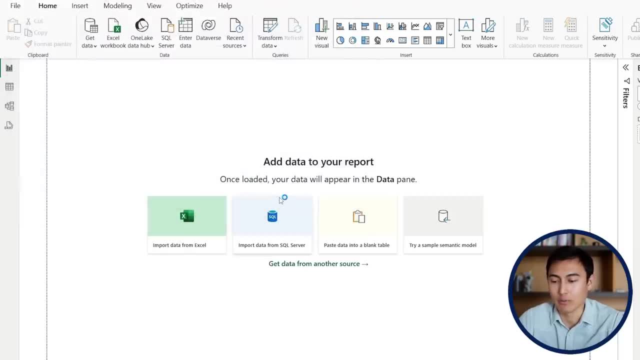 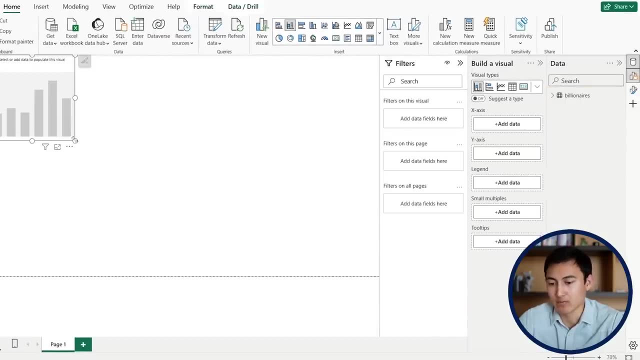 CSV and I'm just going to select it, click on open there and here it is on the side and I'm just gonna load it up. here's the data to the side so I can create some kind of a chart. for example, let's suppose I put one in here which is going to be for all of the billionaires. one's going to be. 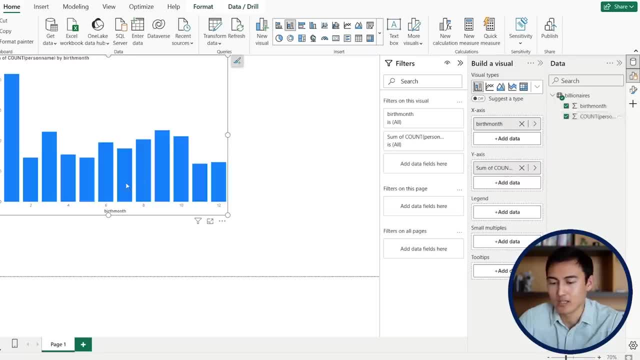 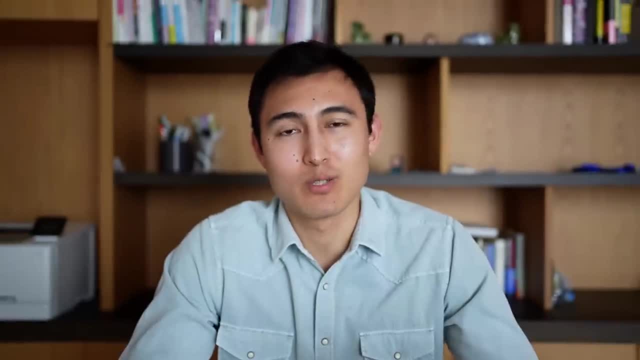 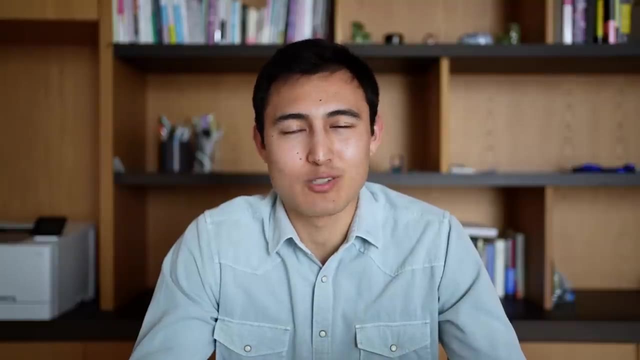 say on the x-axis and the other on the Y. so you can see here that the month of January is definitely the dominant one for becoming a billionaire. also, it is worth noting that there is a way to create a live connection, but maybe that's for another video. overall, this should give you a good 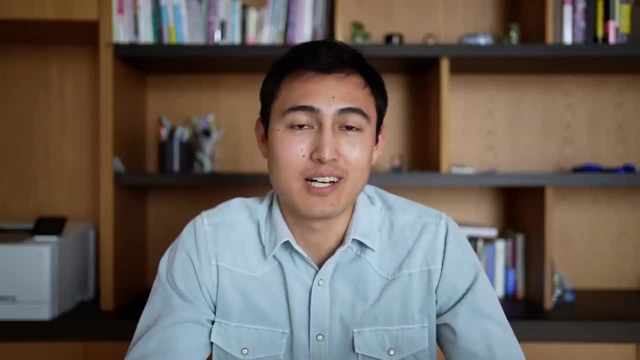 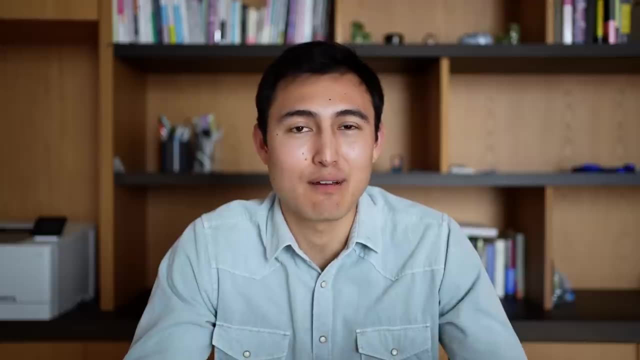 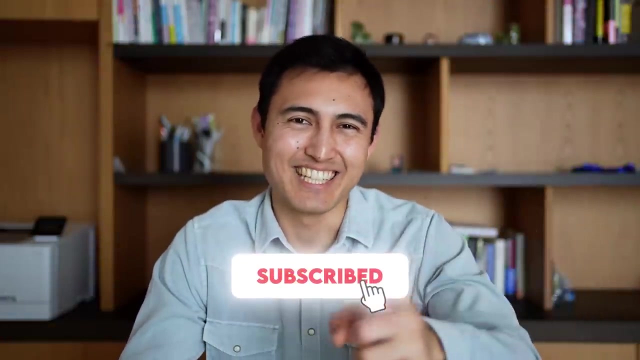 introduction to sequel. that said, there's obviously a lot to learn, like working with multiple tables, using joins, sub queries, window functions and a lot more complex stuff which you can learn in our course over here. so if you like this video, hit the like and subscribe for more, and I'll catch you in the next one.